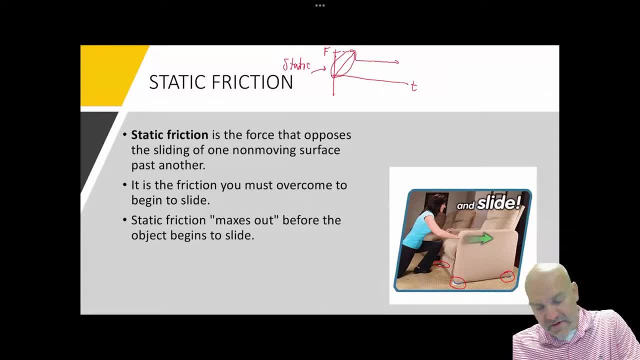 And so this would be our static portion of the graph, and this part right here is actually the kinetic portion of the graph. okay, Now, in most cases, the static friction is greater than the kinetic friction, So Fs is going to be greater than Fk. 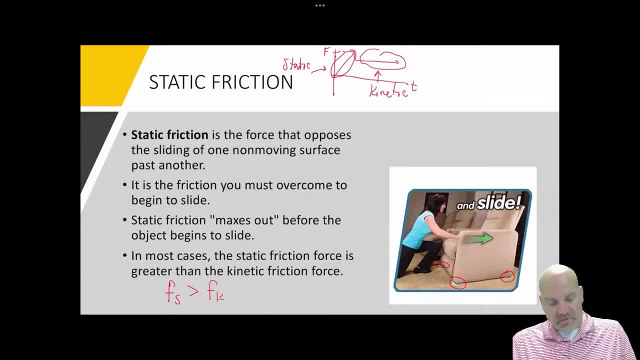 Sorry, lost one of my bullet points. okay Again, remember, we're looking at the interaction and that's what I'm saying In most cases, because everybody's like, oh, but what about here? This static friction was less than the kinetic friction. 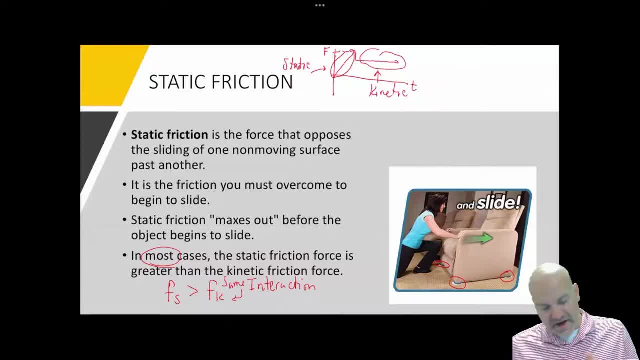 Well, you've got to make sure it's the same interaction, right? So, for the same interaction, Fs is going to be greater than Fk. Now what happens? What happens is the equation for the coefficient is or, excuse me, for friction- is the same. 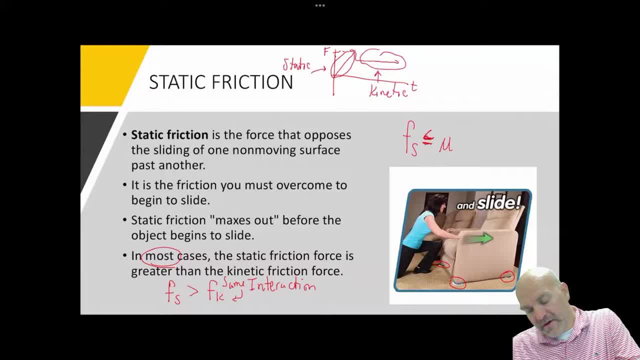 but the difference is, with kinetic friction, all the time we put an equal sign, but for static friction we'll put this less than or equal to sign, okay. So basically that's telling us that if we're less than the static friction, 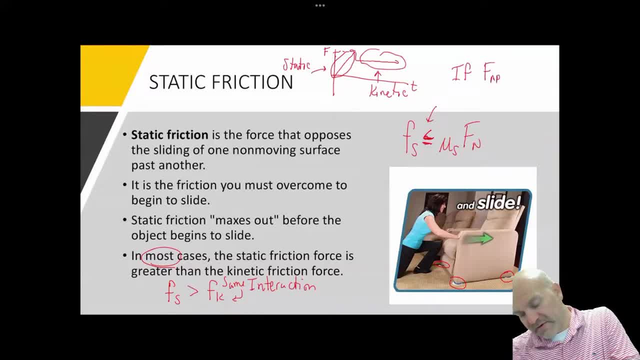 the object is not going to move. So if our applied force is less than Fs, the object will not. excuse me, can't spell this morning, will not move, Can't write either, right, So it will not move. So if I know that I have to have at least 50 newtons of force to begin the object to slide, 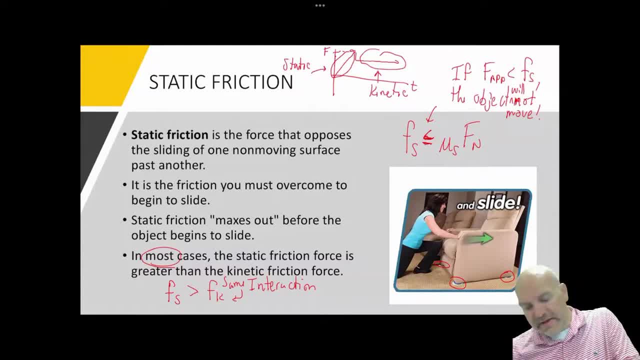 and I'm only pushing with 30, there's no motion? okay, It's not moving. And in these questions our acceleration will be zero. okay, Because we're not accelerating the object yet. right, We're trying to get the push. 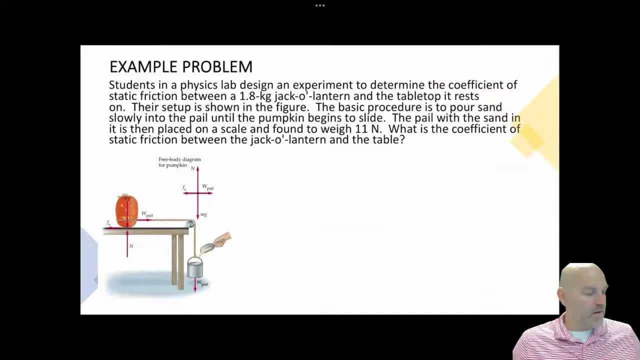 Okay, Constantly. So let's look at a static friction problem. okay, And this is an Atwood machine problem, okay. So this says students in physics lab design experiment to test what is the coefficient of friction with the pumpkin on the tabletop. 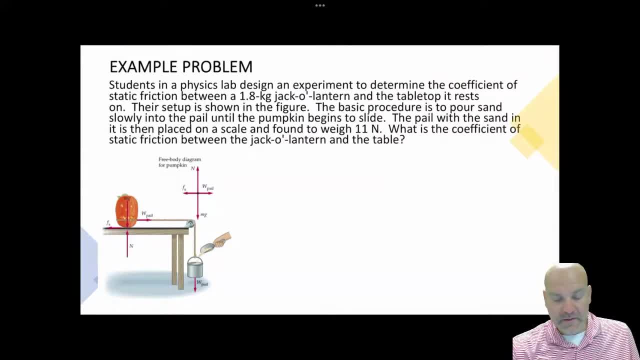 You can see they set up the setup in the figure. The basic procedure is to pour sand slowly into the pail until the pumpkin begins to move. The pail with the sand in it is placed on a scale and found a way 11.. 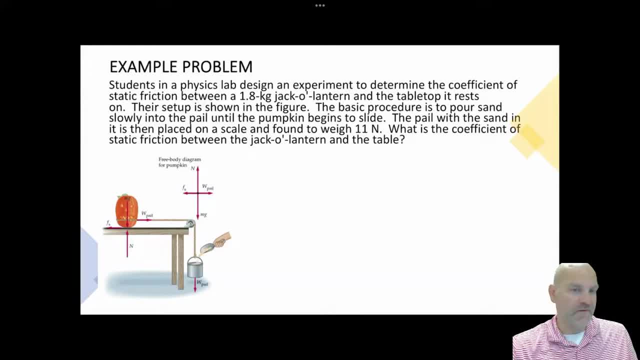 11 newtons. What is the coefficient of static friction between the jack-o'-lantern and the table? Perfect, because this video is being created around Halloween. We're about four or five days, six days away, seven days away, okay. 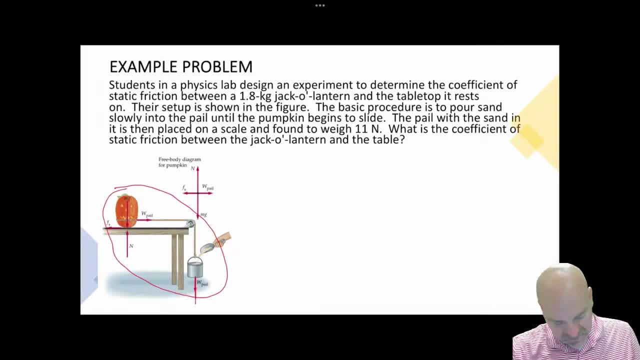 So I'm going to treat this as a single object, right, And so what forces are pulling this object? It's going to be the friction right And the friction on the table and the hanging bucket, And so I'm going to do my free-by diagram. 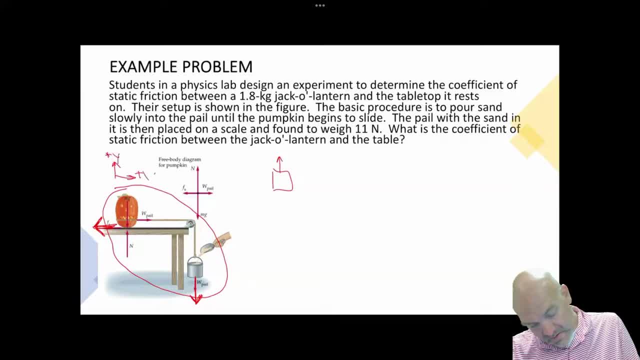 So this is kind of weird. Okay, so I got plus my positive x, But what happens is the coordinate system has to follow through the pulley, And so my positive x actually points down. So this: the weight of the pail is actually in the x direction, as well as the friction. 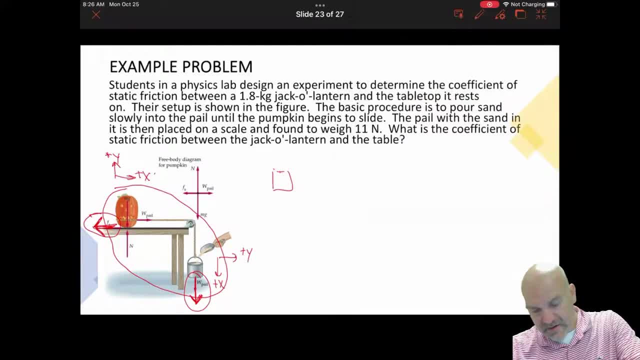 So let me go back and fix my free-by diagram to show that these are going to be in the x direction. So My positive is going to be the pail right, So FG pail, And then I'm going to have my friction okay on my surface. 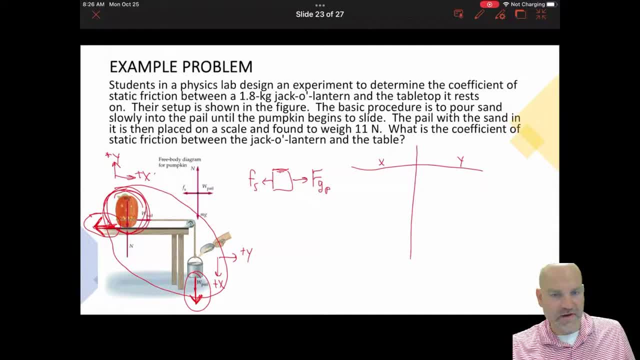 Now what happens is, I do need to know what is the normal force here, Because when we do the coefficient friction, okay, we need to know that normal force. So if I do that real quick, it's going to be. in fact, they give you the whole free-by diagram. 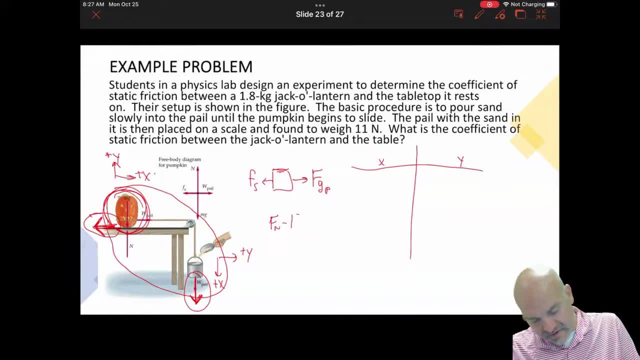 They give you the free-by diagram for everything, right, And so it's going to be: FN minus FG equals zero. So FN equals FG, which equals MG. So that's normal, That's usually pretty standard. And so now my pumpkin, or my motion right of the system, is just going to be in the horizontal direction. 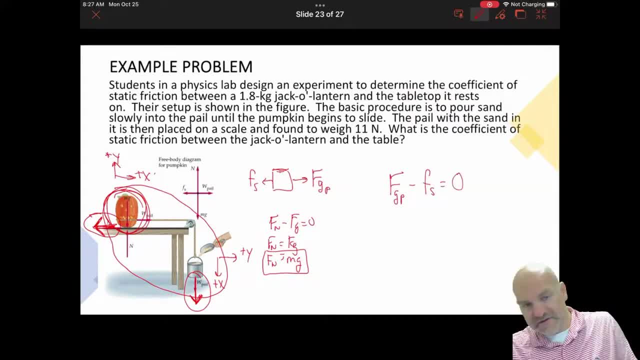 So I'm going to have FG pail minus friction, And so FG pail equals FS, And so now I can just start substituting in. I got the weight of the pail. Weight is MG, And so this is going to be here. 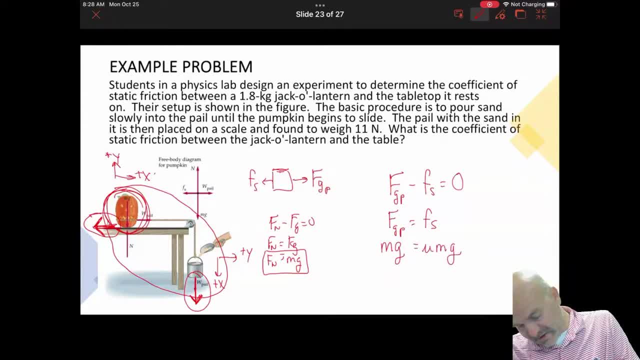 Apologies, This is going to be yeah, And so this is going to be mu MG Teachers. for those of you who are in G Hall, they see this. It's been recorded and help is on its way. Thank you. 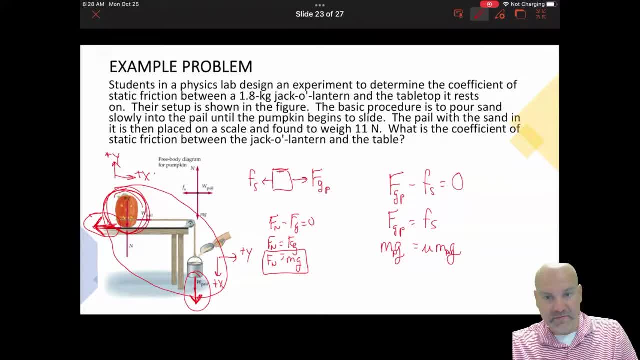 Have a good day. So we do need to distinguish that the mu MG mass is actually the pumpkin And then the FG is the pail. Okay, So we can't cancel those out, but we can't cancel these Gs out. And so I get: the mass of the pail is going to be mu times the mass of the pumpkin. 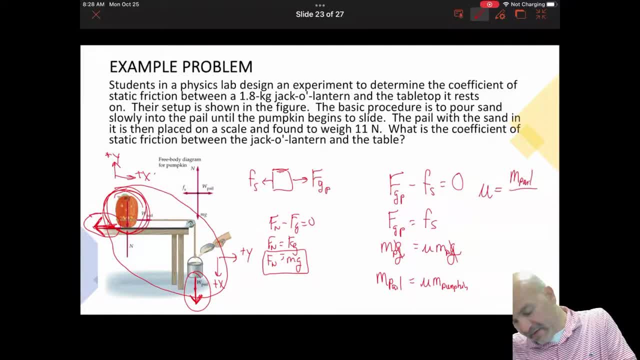 Okay, And so my coefficient of friction is going to be mass of the pail. So I get the mass of the pail divided by mass of the pumpkin, And so that's going to be So. I got to find the mass of the pail. 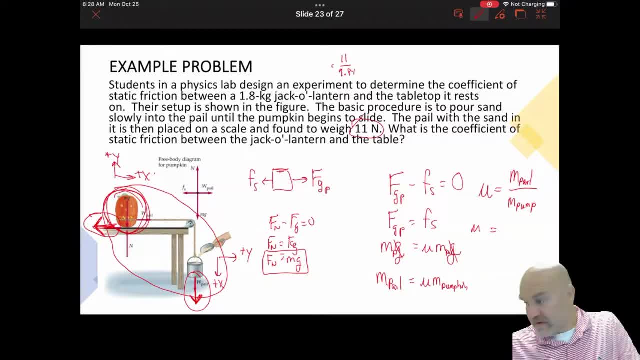 Right. So the mass of the pail is going to be 11 divided by 9.81.. Or here's what I can do. I can, So let's do this. So let's not cancel out the Gs, Right. 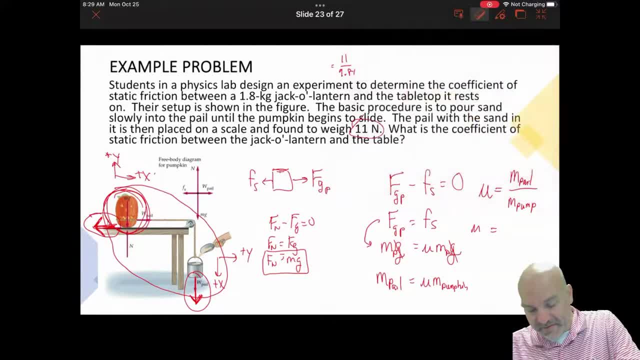 Because it's going to help me. I can use the equation, Or I can use the numbers That are given to me. All right, So let's change this up a little bit. So if I go way back here, I'm going to say this is going to be the force. 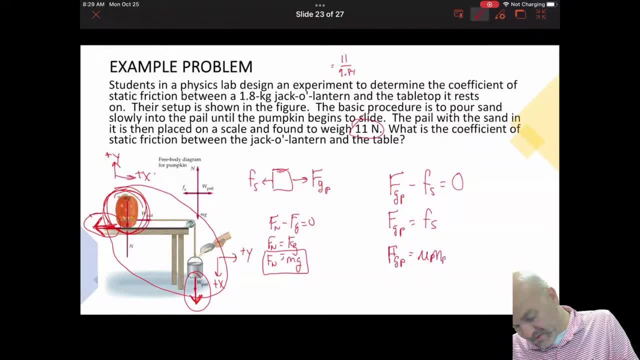 The weight of the pail is equal to the mu times the mass of the pumpkin, times G, And so my coefficient of friction is going to be mass, The sorry I keep messing this one up. It's going to be the Weight of the pail divided by the mass of the pumpkin, essentially the weight of the pumpkin. 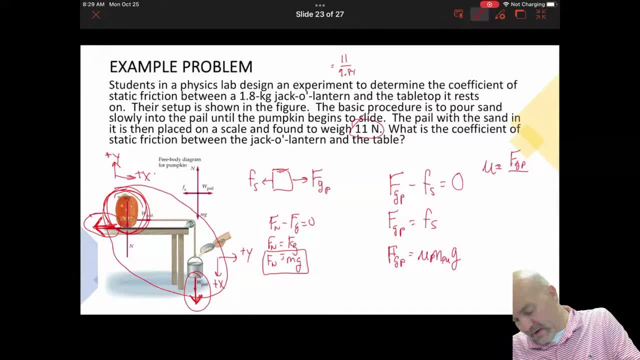 Right, So it's going to be 11 newtons divided by 1.8 times 9.81.. And that's going to end up being a coefficient of friction of 0.623.. Okay, So how do we So this is a static friction. 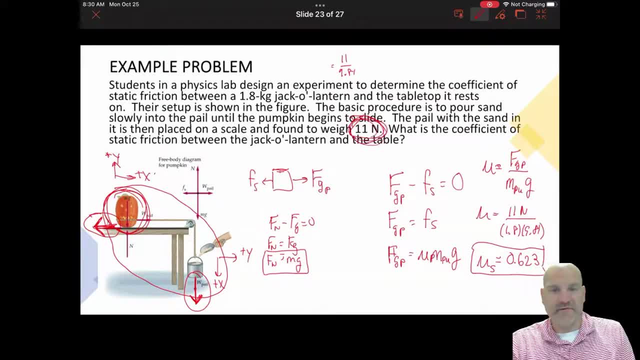 Again, I apologize for the Confusion here, But if I want to use the number that they give me, which for the pail is 11 newtons, I need the. I can't cancel out the the G value, because then it becomes. 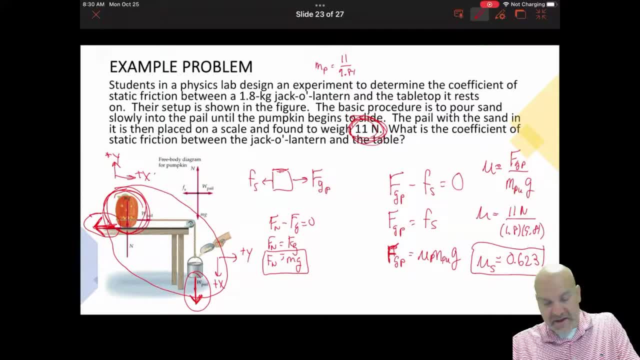 Right, Then I have to go back and add a step of finding what the mass of the pail is by doing 11 divided by 9.81. And then bringing that back in. But if I want to use the numbers given to me, 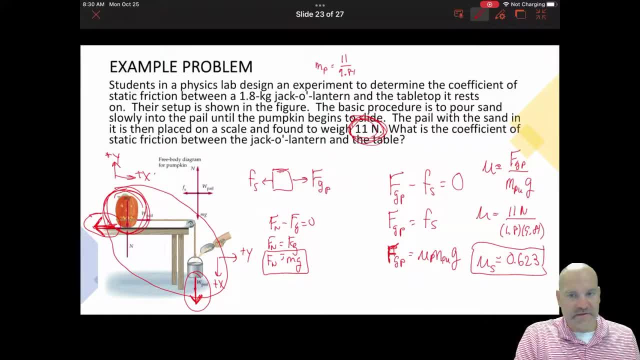 Right, I can just simply not cancel the G's out and find the weight of the pumpkin, Because that's essentially what what we're looking for There. Okay, All right. So again, we're going to keep our journey going. We're going to move on to the videos like connected objects, which is actually what this is.